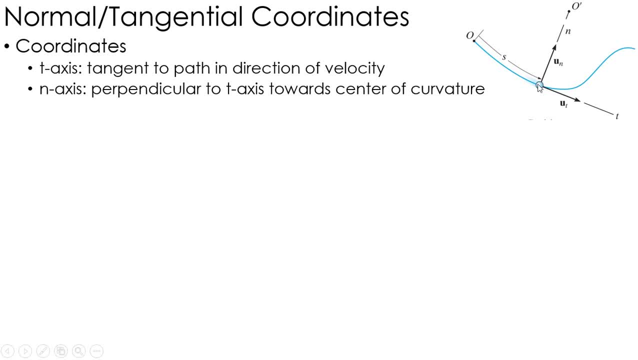 be defined as tangent. that's where the t comes from, tangent to the path, in the direction that it's moving, in the direction of the velocity. The n axis is perpendicular to that t axis and pointed towards the center of curvature. okay, So in this plot here, curving like 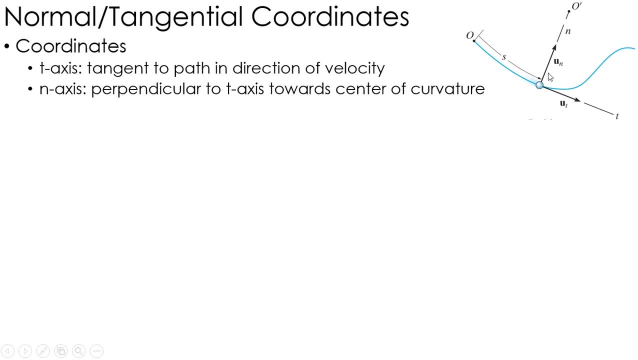 this n points towards the center of that curvature, towards the center of what would be a circle. okay, t is tangent, n is normal to the tangent okay. So once we define that, we can go ahead and define our velocity and our acceleration, as we've done before. So 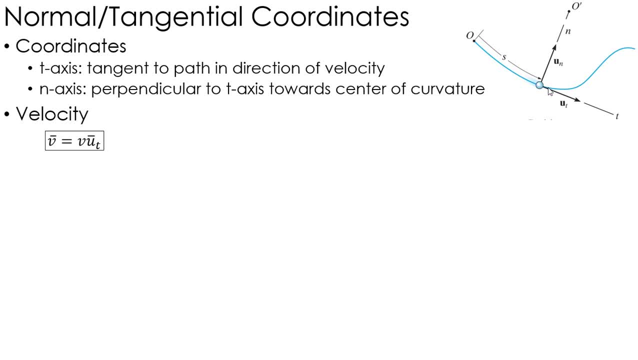 by definition, the velocity is simply the speed v in the direction of the tangent to the path, which we're going to call u sub t, u being the unit vector in the t direction, And that's basically just the definition here. Now, in order to do the acceleration, we have to take a time derivative. 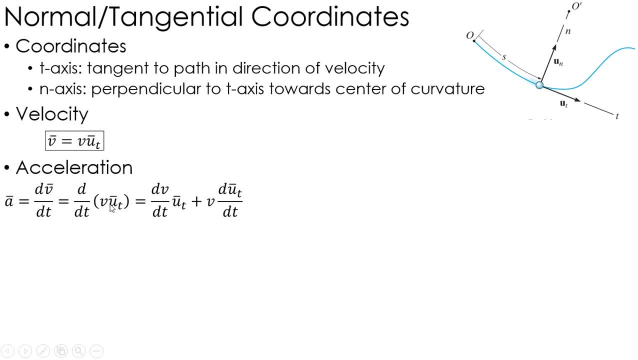 of that velocity, which means I have to take a time derivative of v u t. Now when I take that time derivative, I get dv dt times the unit vector plus v times the time derivative of the unit vector. Now here's the thing: That unit vector changes with time as opposed to with. 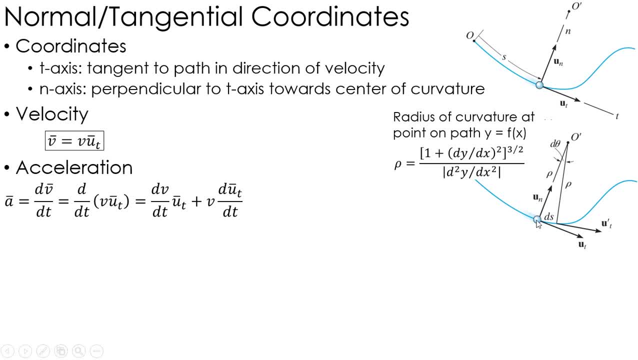 rectangular coordinates. As I move around that path, right u t changes in direction. Therefore I can't just throw that away, call it zero, because it does change as a function of time. So at this point, if you just want to skip ahead, get the final answer, that's. 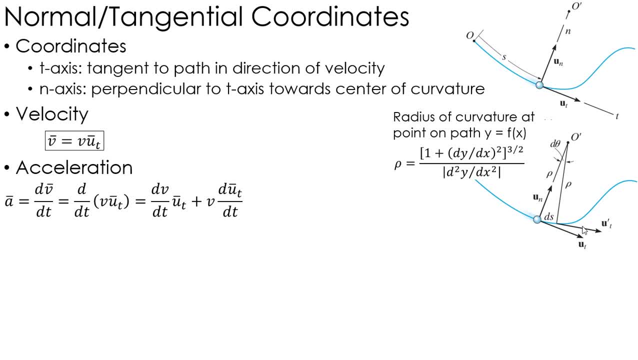 great, We're going to go through the derivation to get the acceleration in the normal and tangential directions. okay, To do that, we need to follow this, And first we should define the radius of curvature, which would be, you know, for these two points: where would the center of? 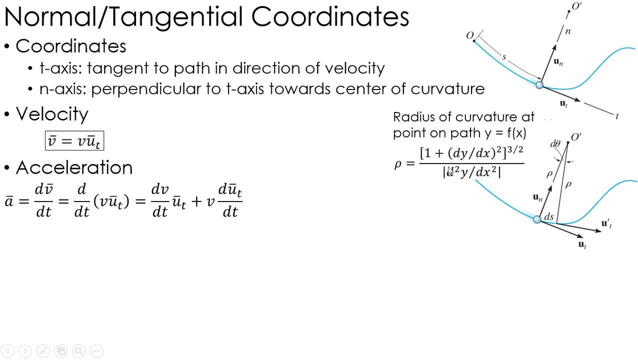 the circle be: What was the radius away? If you look in any calculus book, it'll have this. Let's just throw it up there, so you have it. If you have the equation for the path, you can find the radius of curvature at any point. okay, So? 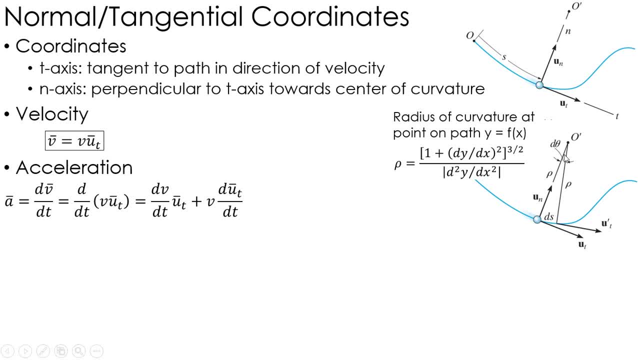 again, I move from here to here some position d s through an angle of what I'm going to call d theta, at a radius of curvature of rho, which I can find from this. Therefore, that arc length, or d s, is simply that radius of curvature rho times d theta. Now, of course I can divide this. 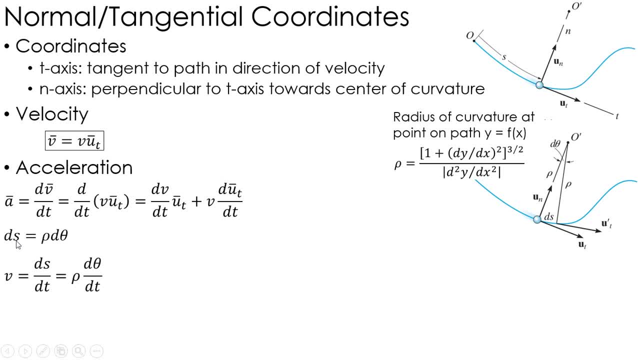 by d t right, which would be d s d t, d theta d t. okay, And I hope it's obvious that d s d t equals the velocity right And, by definition, d s d t equals the velocity. okay, And that's going to. 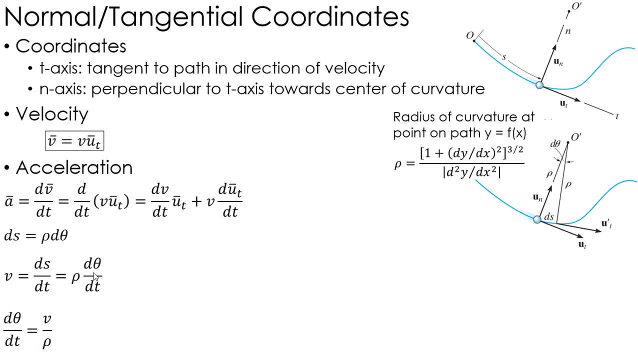 equal rho times d theta d t. okay, So, rearranging a little bit, I can get d theta d t equal to the velocity divided by the radius of curvature. okay, So again, the change in angle as a function of time is defined as the velocity divided by the radius of curvature. 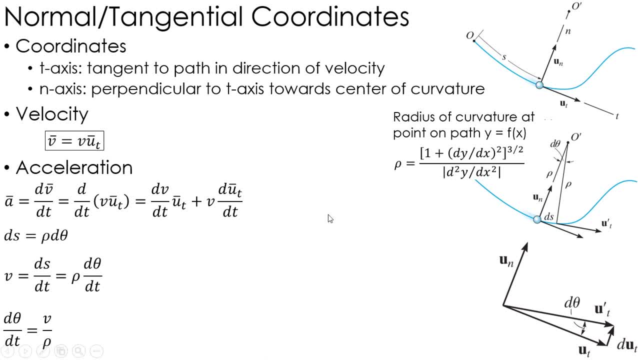 Now I can also look at something. this because, again, what I'm basically trying to find is find the time derivative of my unit vector in the tangential direction. So the change in the unit vector is given by this little vector right here. right u t is pointed in this direction, u prime. 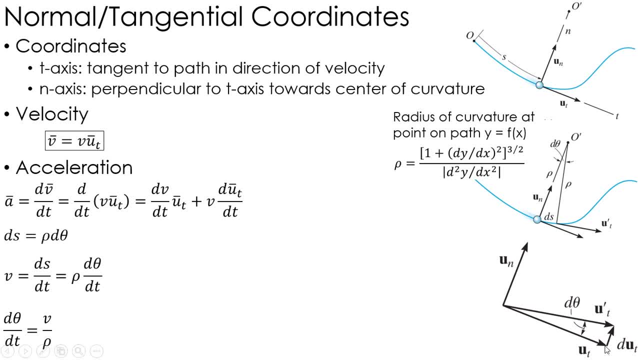 t is pointed in this direction. So I have this little infinitesimal change in the unit vector, okay, And that is equivalent to to the magnitude one, if I think about this as an arc length, just like I thought about d s. 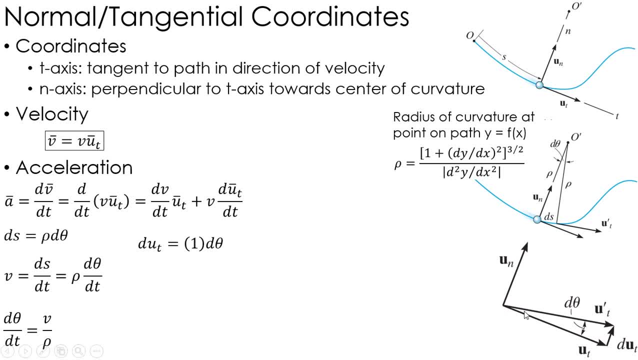 right, This radius is one, because this is a unit vector. okay, Times the angle d theta right. So d u t is just one times d theta. Therefore, okay, I can write this in vector form. okay, Which is what I want to find. I want to find the time derivative of that vector. 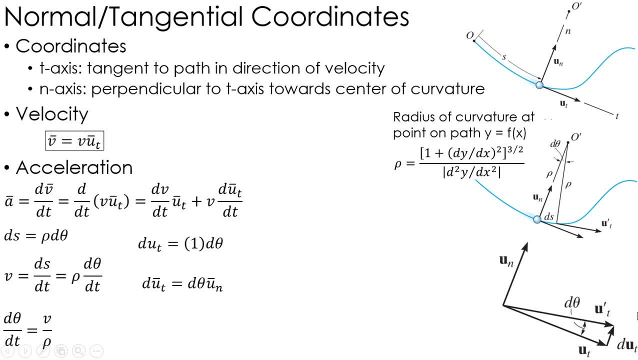 okay, So I know the magnitude is just d theta and also that that vector is pointing in the same direction as the unit vector right. This is in that direction, So I can write the d u t in vector form as just d theta. 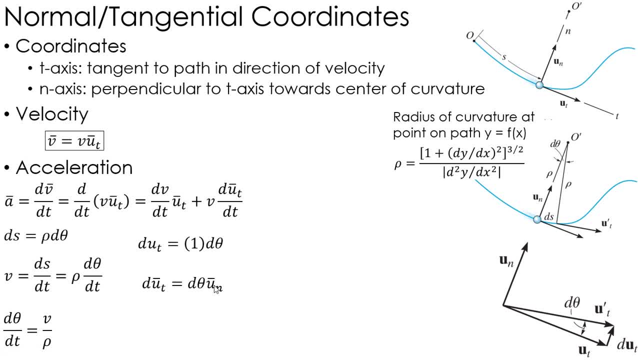 times: u in the n direction, u sub n in the normal direction. Taking a time derivative of this, I can get again what I'm looking for: d u d t right d u d t equals d theta d t. 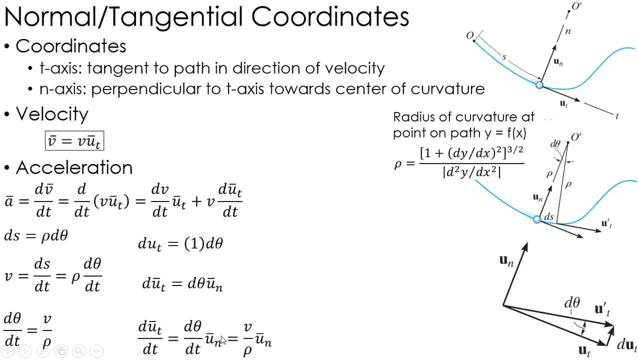 u? n Again, just basically dividing this equation by d t. Now, over here again, I found d theta. d t is just velocity over rho, so I can plug in that into here. So I can find that the time derivative.